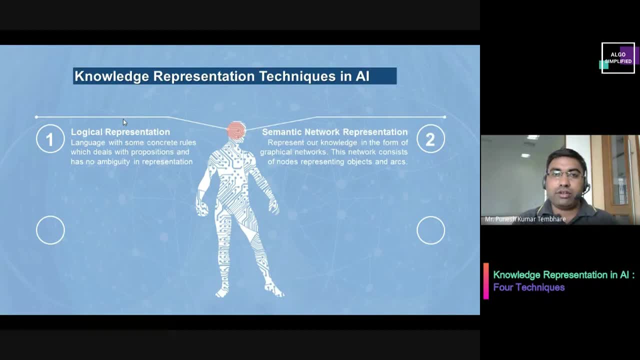 representation. Second one is semantic network representation. Third technique is frame representation and fourth technique is production rules. So in earlier classes how to represent the knowledge is by logical representation, semantic network representation and production rules we have already discussed, and in today's class we have to go for the knowledge representation. 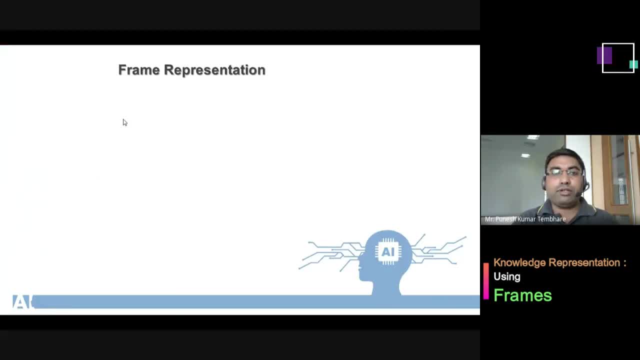 by using frames. So whenever we are representing the knowledge with the help of frame representation, at that time this representation is more structured as compared to the previous techniques is concerned. Frames are generally organized into hierarchies or networks of frames. Lower level frames can inherit the information from the upper level frames in 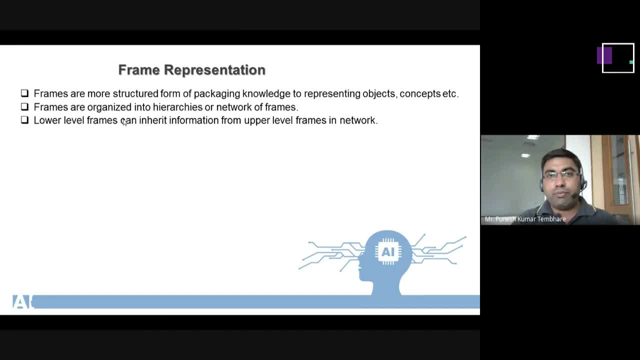 the network. So generally when we represent knowledge through frames in network form, at that time we will make some frames class frames, or some frames class frames or some frames subclass frames, So all the subclasses can inherit the information through their superclasses. And generally when we show the inheritance mechanism, at that time nodes are connected. 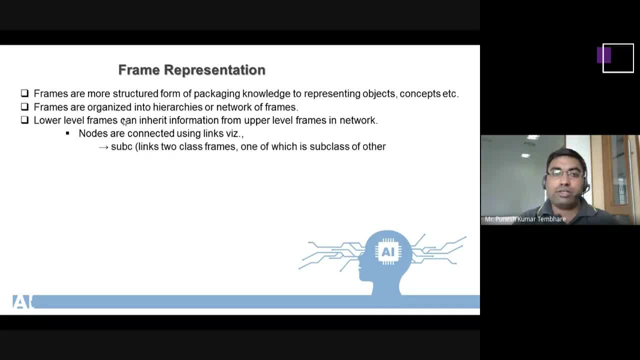 using the links, and these links will be generally in the form of relations, and the relations can be of different types. The first relation will be a subclass, Then second relation will be of kind is a. So each particular connect, a particular instance of a class frame. Third type of relationship: 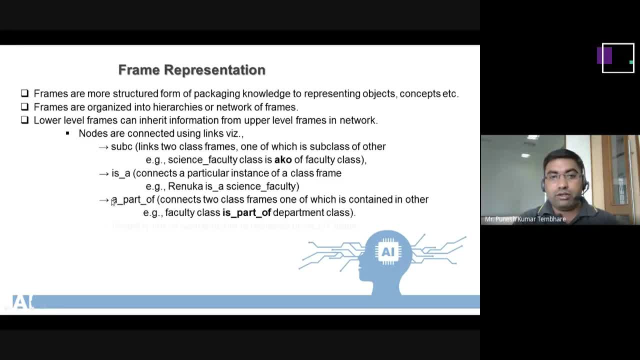 that can be. that will be a part of And fourth type of relationship frame. that will be the proper tingling In this way, generally through frames. if we are representing the knowledge, then while representing the knowledge, frames are represented in the form of nodes and in 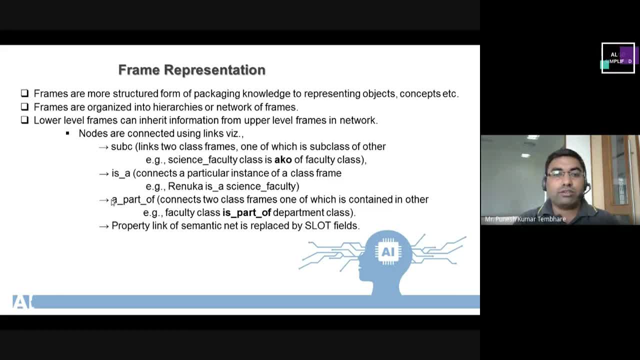 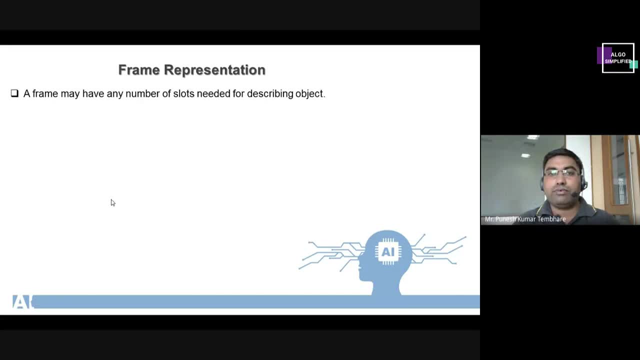 multiple frames. we are giving this type of relationship Now. a frame may have any number of slots needed for describing the objects. Example: faculty name may have name, age, address, qualification. Generally we will call them slot names. So, while representing knowledge through frames, we will make multiple slots and we will put value in the slots. 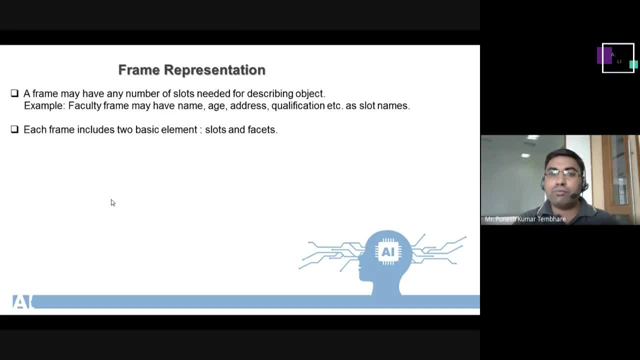 So whenever we talk about any frame, there will be two elements in that frame. First element will be slot and second element will be facet. Now, what will be slot? So each slot may contain one or more facets, which are generally called as fillers. 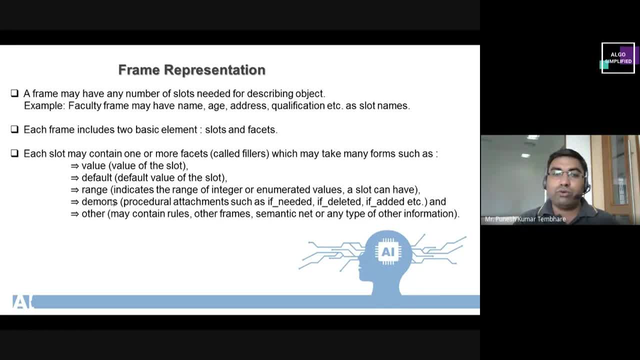 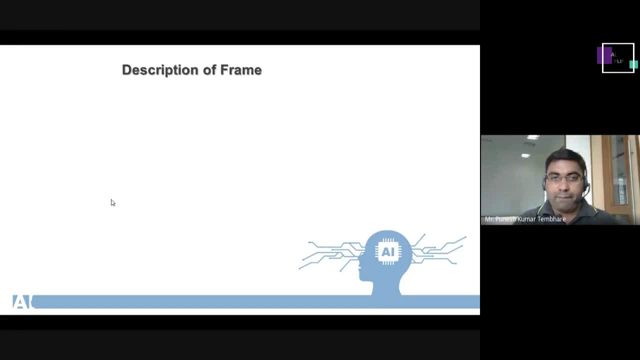 Which may take many forms, such as value, default value, range, demands or other information. Now we have to go for the description of a frame, So each frame represents either a class or an instance. Generally, information can be represented in the form of a class or in the form of an instance. 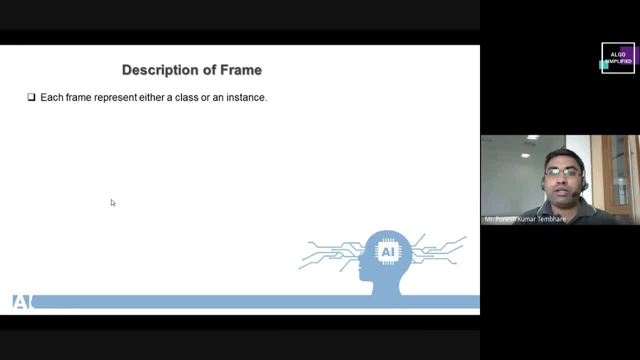 If there is information representing a class, then we have to formulate a class frame And, for instance, the frame we will make will be the instance frame. A class frame represents a general concept, whereas instance frame represents a specific occurrence of the class instance. 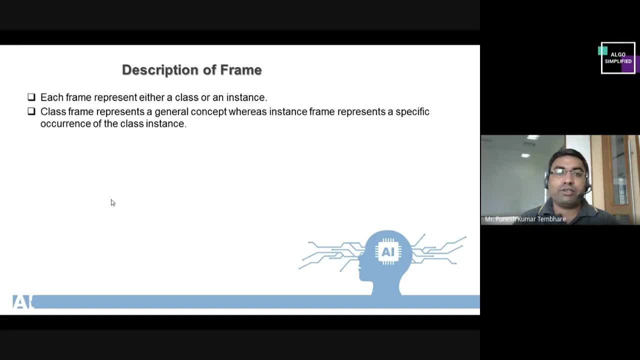 If we want to represent general information, then generally we will represent it through a class frame. But if we want to represent particular instances, then at that time we have to go for the instance frame. Class frames generally have default values which can be redefined at lower levels. 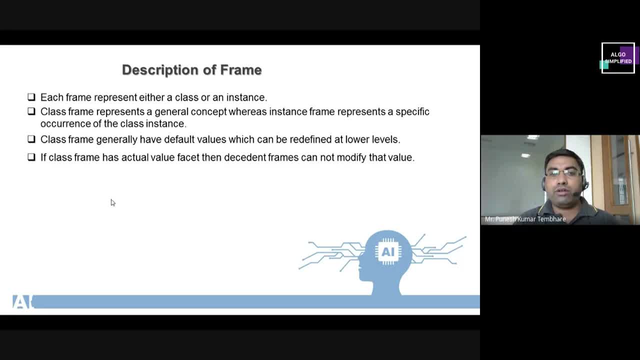 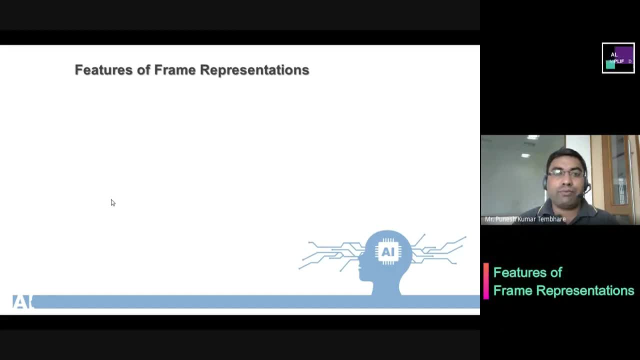 If a class frame has actual value facets, then descendant frames cannot modify the value. Now we have to understand The features of frame representation. Frames can support values more naturally than the semantic networks. Generally, if we talk about frames, then frames are a natural way to represent information. 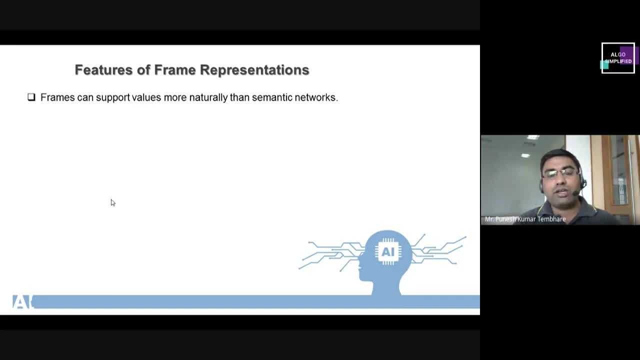 Why? Because when we represent knowledge through frames, we are following an object-oriented mechanism. here, Frames can be easily implemented using object-oriented programming techniques. So generally, the way we represent knowledge through frames is that we represent information by following an object-oriented mechanism. 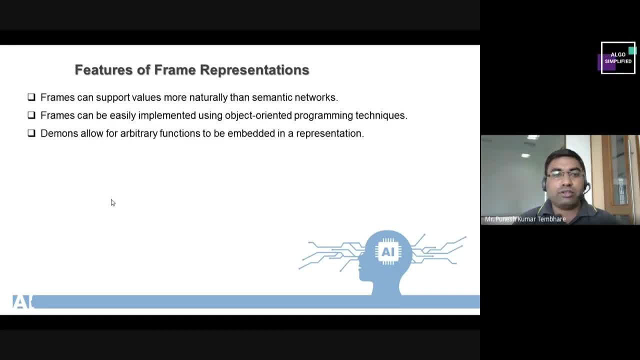 Demons allow for arbitrary functions to be embedded in a representation, But a price is paid in terms of efficiency, generality and modularity. Inheritance can be easily controlled, Why? Because we are using the entire object-oriented mechanism. So here we have to understand the example of one frame. 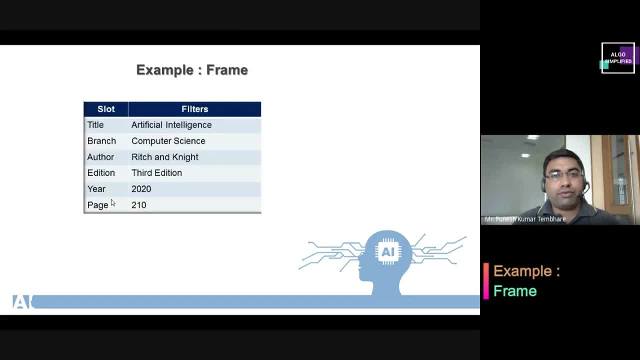 So here we have one frame. This frame is representing the information regarding one book. So we have slots and various filters. The slots are title, branch, author, edition, year and page, And the corresponding values are entered in the filters. 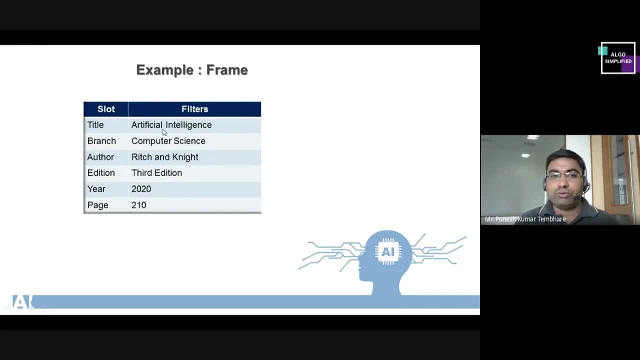 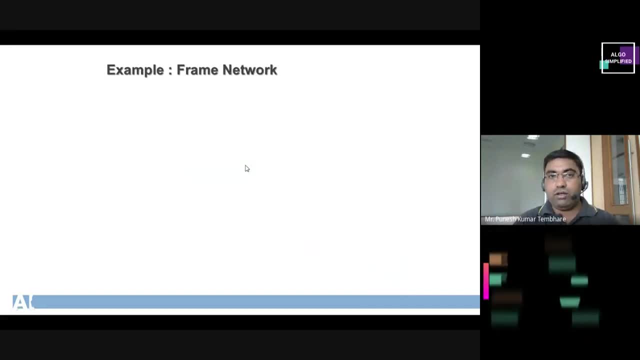 If the title is artificial intelligence, the branch is computer science. In this way, we can represent the information regarding one book In the form of a frame. Now we have to understand the frame network with one example. So here we have one frame. 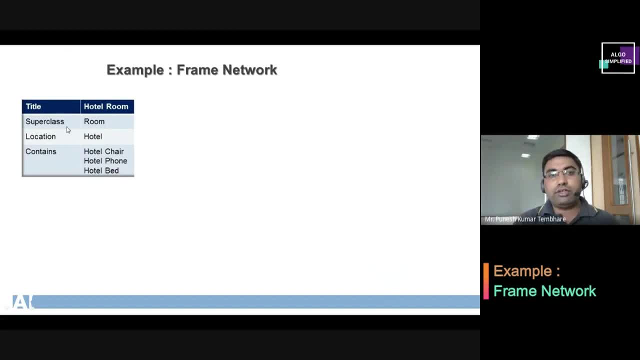 And this frame is generally representing the information regarding the hotel room, And that's why the title of the frame is what a hotel room is. Now, the frame named hotel room is a super class of the frame. That is what a room class is. 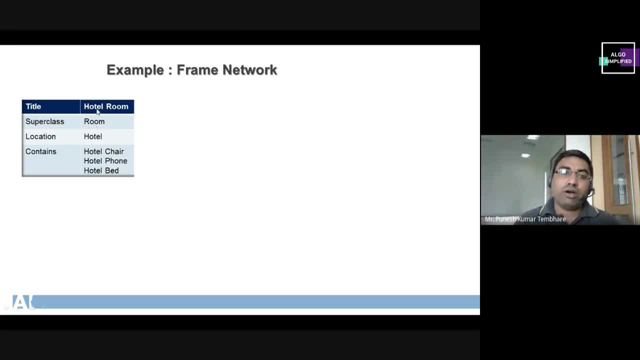 So somewhere there will be a frame named room And it will have a subclass That will be the hotel room. Then we have another slot, Location and contents. So in the location we have kept the hotel here And in the contents- hotel chair, hotel phone and hotel bed. 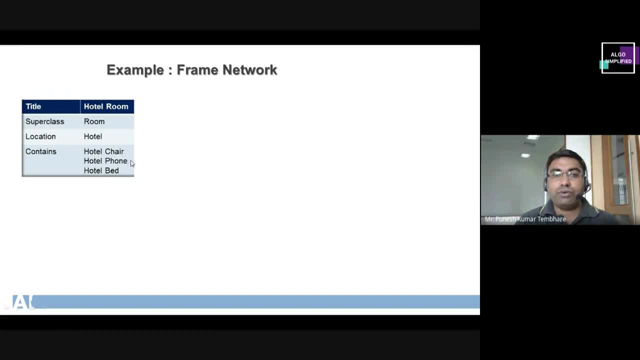 So now we have information here That is in the form of chair, phone and bed, And that's why now, Moving forward Only with the help of a single frame, we cannot represent the information. So if we have multiple information, 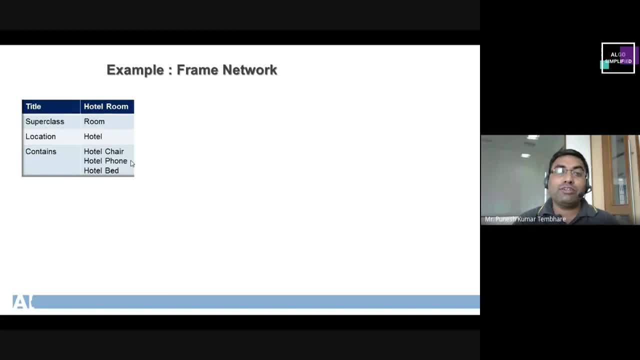 So how is that multiple information related to this frame? How is it related to this frame? We will show all that through the relation or through the network, And that's why now we have to go for the formation of a frame network. So very first, 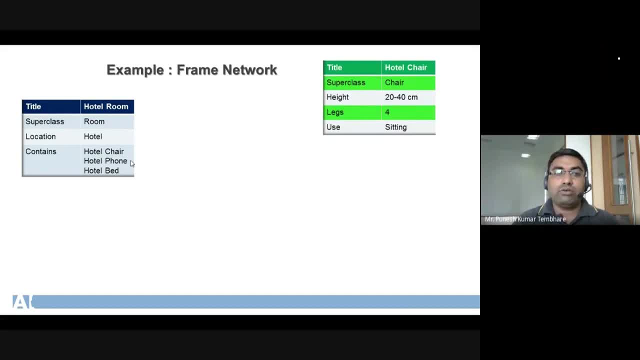 Now, here we have the next frame Hotel chair. Why? Because you can see, in the frame named hotel room We had stored this information, That is, hotel chair, And now we have to store information in detail about this frame. That's why the frame named hotel chair will be made. 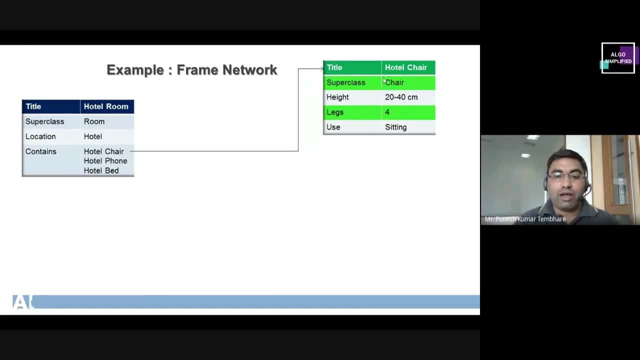 And we will show the relationship between them here Now, what will happen inside the hotel chair? So, if we talk about the hotel chair of this particular frame, So this is what, once again, a subclass And subclass of which frame, Subclass of frame is a chair. 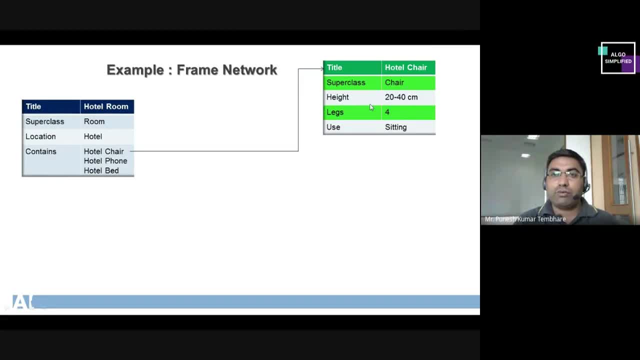 So here there will be a class named chair, There will be a super class of this particular frame, And later we have kept the slots, Height legs and corresponding values. Next we have next frame form. Here we have This frame is a hotel phone. 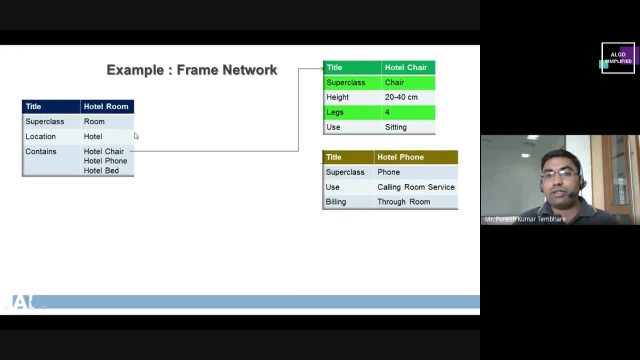 So hotel phone is related to the hotel room And that's why there is a network formation. Then we have next frame That is a hotel bed. Then we have next frame That is a title mattress. Now you can see here Inside the frame named hotel bed. 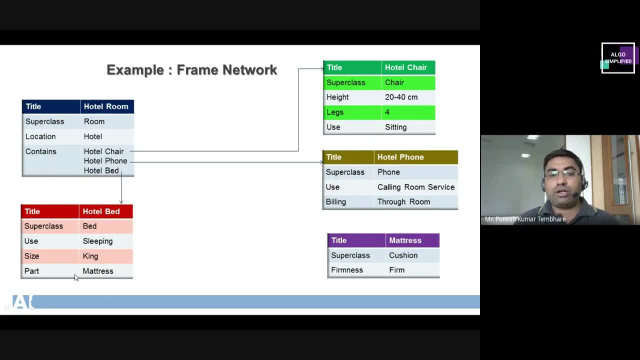 We have stored information named mattress. So then, if we want to give the details of this, So in this way we have to formulate the frame network, So, generally, through frames, If we want to represent the knowledge, Then all the knowledge can be represented through single frame. 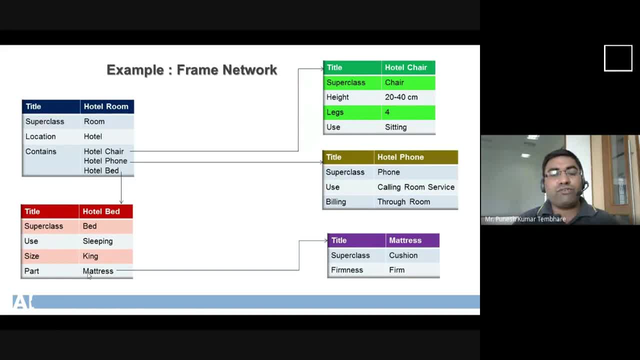 So for that we have to go for formulation of various frames, And when we make a lot of frames, Then some of the frames will be class frames, Some of the frames will be instance frames, And these frames will be connected to each other. 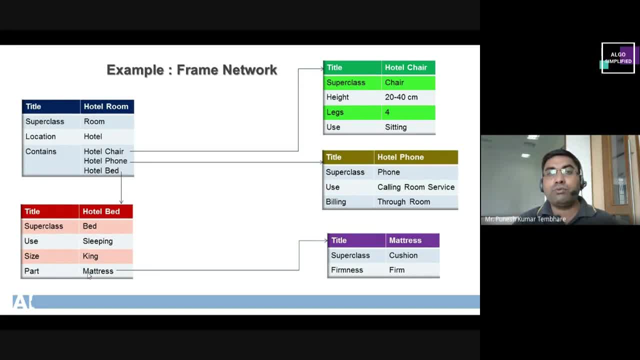 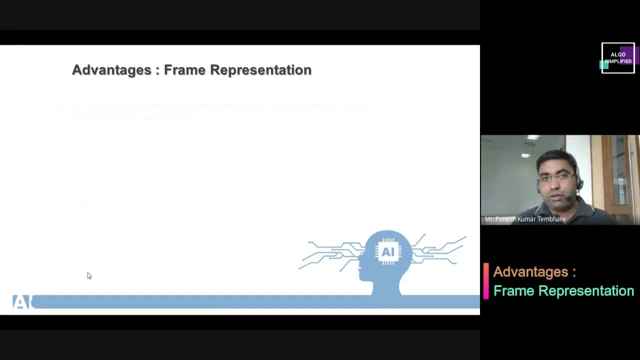 Their frame network will also be with us, Which we have seen through this example. Now we have to understand The advantages of frame representation. The first advantage is The frame knowledge representation makes the programmer Easier by grouping the related data. Actually, we use the mechanism of classes and objects here. 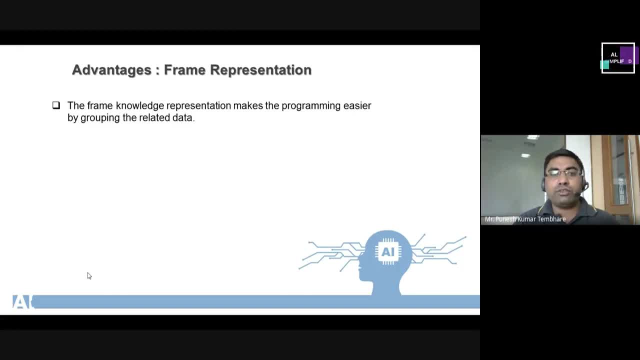 And that's why if there is some related information, Then we can make a group of related information And we can represent it. So this particular facility is provided In this knowledge representation scheme. Second, The frame representation is covered And it is comparably flexible. 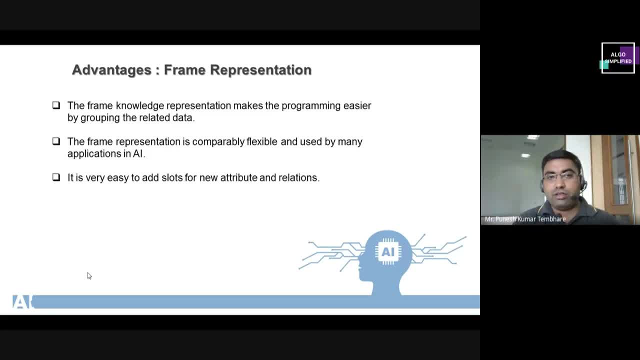 And used by many applications in artificial intelligence. Third advantage is It is very easy to add slots for new attributes and relations. If our attributes increase, Or if we want to add new relationships, Then by simple addition of slots We can easily increase all these things here. 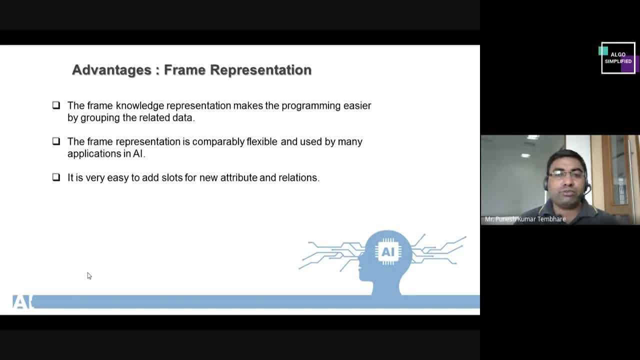 And that's why it is very easy to add the slots For new attributes and relations. It is easy to include default data And to search for the missing values Whenever we are going for the frame representation. Frame representation is easy to understand and visualize.